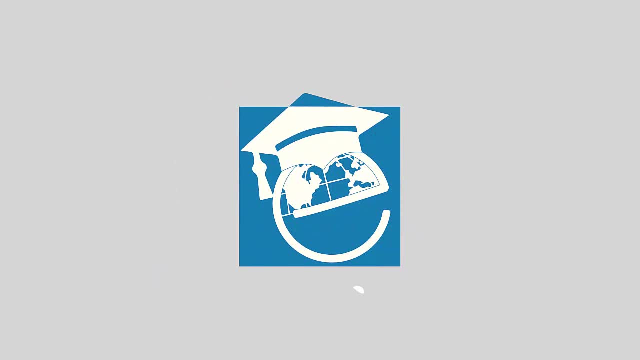 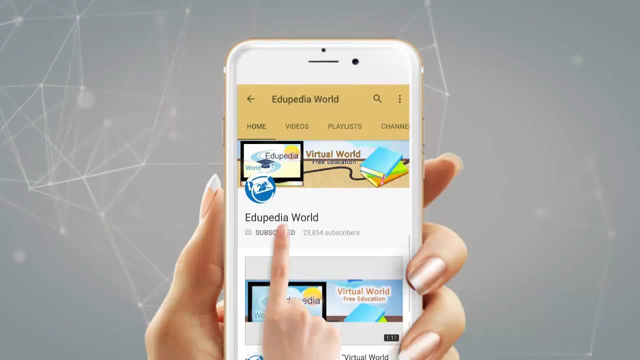 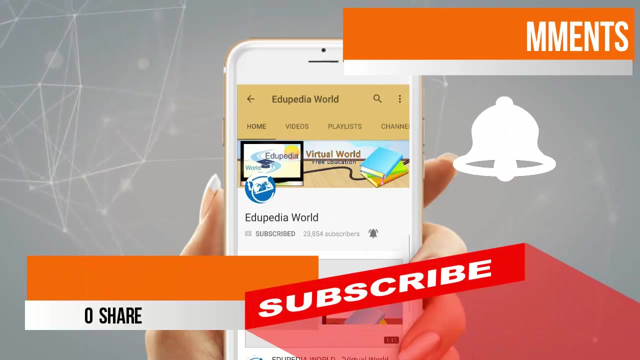 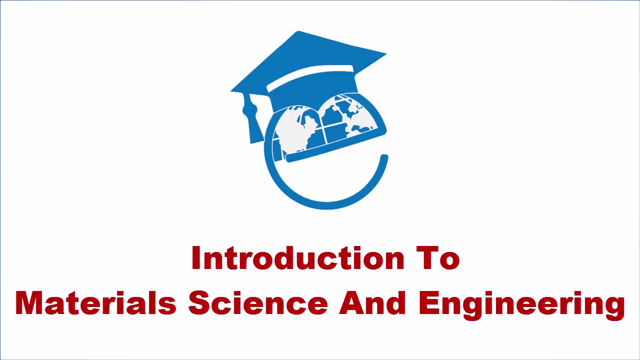 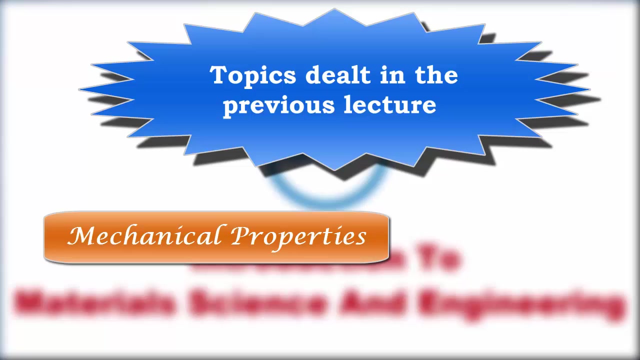 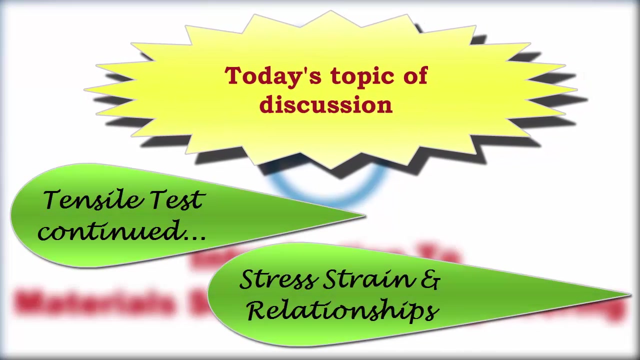 Hi friends, welcome back to Edupedia World. This is the course on Introduction to Material Science and Engineering. Previous lecture we started discussing about mechanical properties and we focused on tensile test. Today we will discuss further about the tensile test and stress strain, stress strain relationship and those things. So to begin with the discussion. 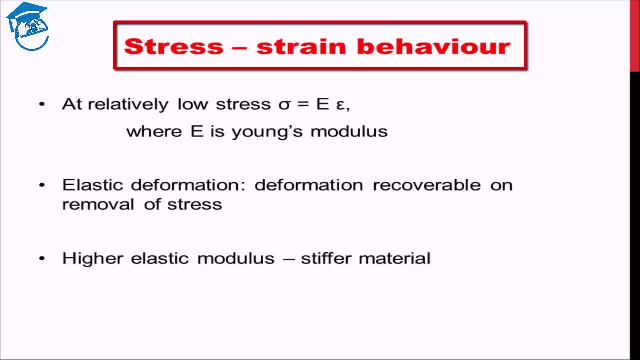 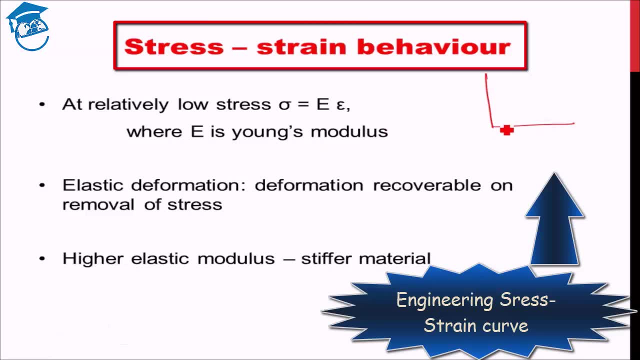 on stress strain behavior, as we saw in the previous lecture that we have. if we plot the engineering stress strain curve, then it looks something like this: right, As we will see in the next slide, that each region has some significance and there is a linear region. 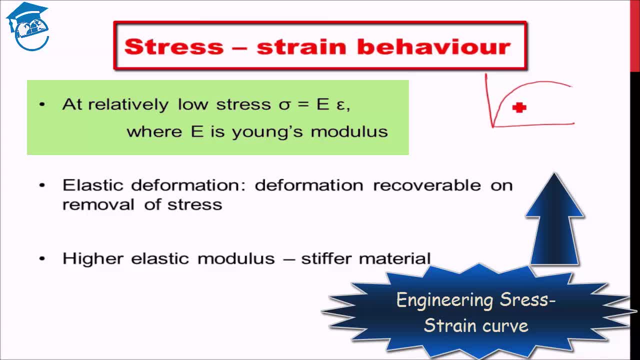 and then non-linear region At relatively low stress. this is the linear region and that region follows the relation similar to Hooke's law. What did Hooke's law say? Stress is proportional to strain right, Or elongation is proportional to force. 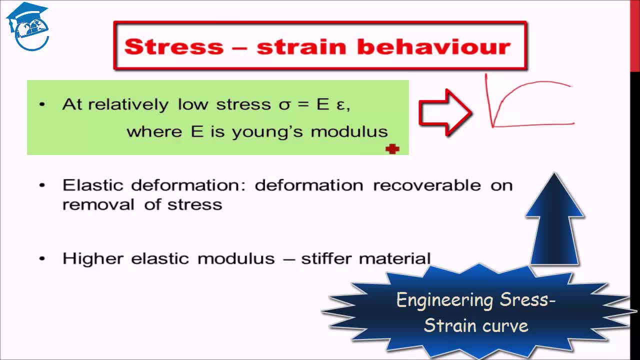 Instead of elongation, is proportional to force. here we have stress is proportional to strain at low stresses, And the proportionality constant that is used to relate stress and strain is known as Young's modulus. This E is Young's modulus, So stress is equal to. 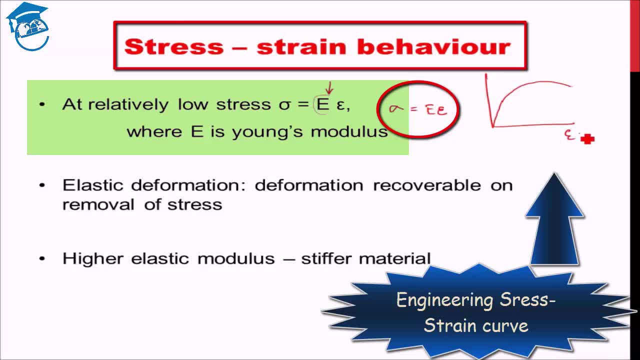 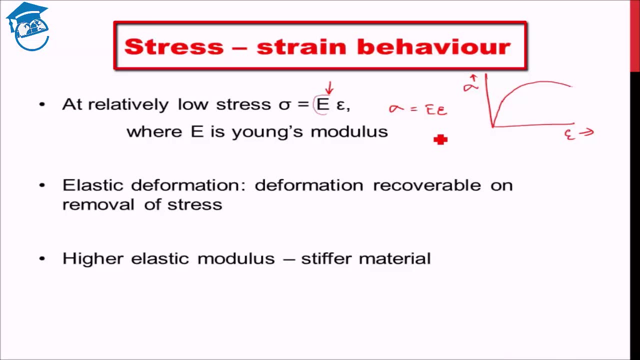 Young's modulus times strain. This is strain, this is stress. As we increase stress, strain increases in the proportionality of Young's modulus. Now there are two types of deformation that is taking place when you deform a material. There is an elastic component of deformation. 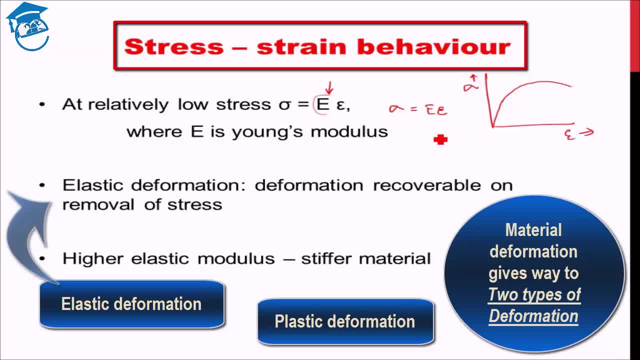 and there is a plastic component of deformation. Elastic deformation is the deformation which can be recovered back on removal of the stress. So if you remove the stress, the elastic deformation is recovered, Whereas plastic deformation is the permanent deformation that you cannot recover back on. 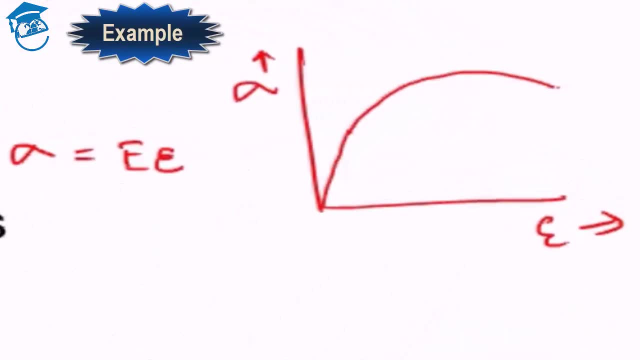 removal of stress. For example, if you stress it till this level and then you remove the stress, what will happen is that the material will come back along this line that is, parallel to this line, parallel to the linear region. Then it will again come parallel to the linear region. Therefore, here you can see that the 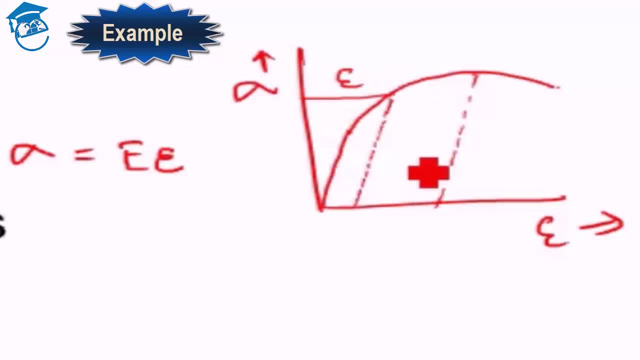 total elongation. is this much right, Epsilon? But actually this much is the elastic deformation And only this much is the plastic deformation. So the elastic deformation is recovered on removal of stress. Plastic deformation is not recovered. This much was plastic which is not recovered and this much was elastic which is recovered. 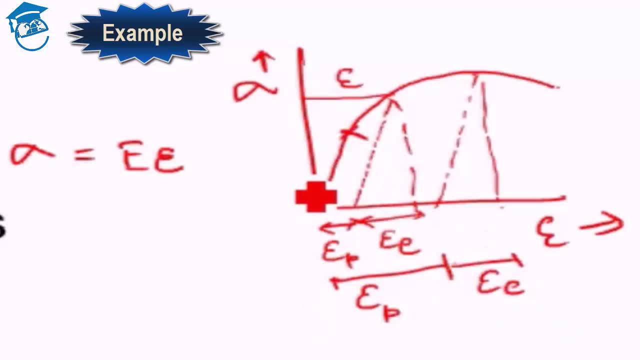 Now, if we remove the load over here, then what happens? It goes straight, it comes straight. So all the deformation till here was of the elastic nature. There was no plastic deformation. So till here the material behaves exactly as a spring. You elongate it, you remove the. 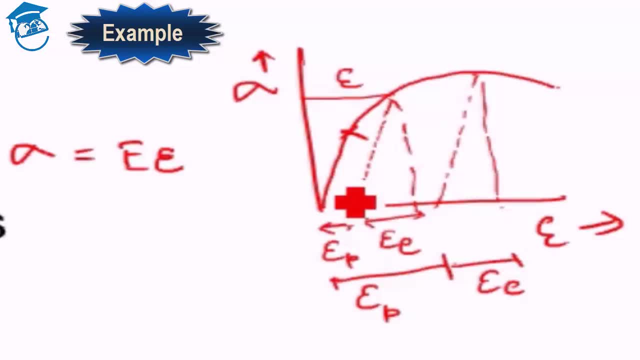 stress. it comes back to its original dimension And this region is known as the yield point. Yield point is the region till where no plastic deformation Beyond that there is plastic deformation. Somewhere you will read it is the proportional limit, But generally speaking, yield point. 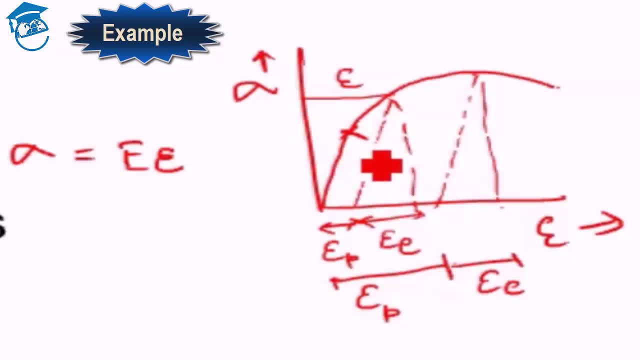 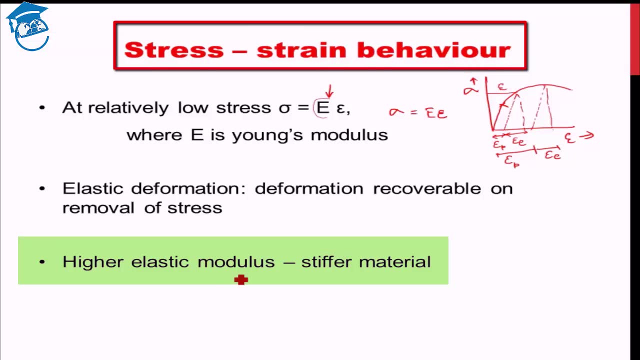 and proportional limit are very, very close. Okay, we will discuss these terms in the next slide. One more important thing: that higher the Young's modulus, that is, higher the elastic modulus, stiffer will the material be. What does this mean? Suppose we have two types. 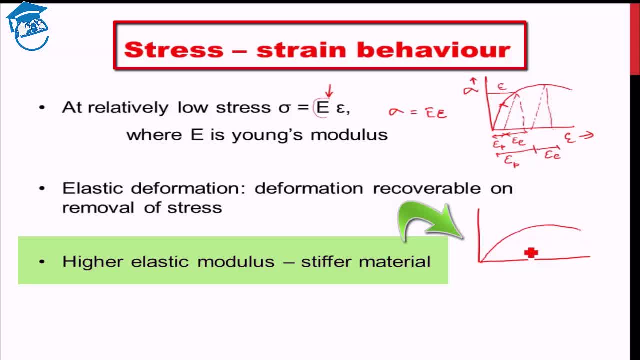 of materials, two different materials. One has a nature like this and another has a nature like this. So till here the linearity. is there? linearity, The Young's modulus for this material. So the first material is this slope right, Whereas the Young's modulus for the second 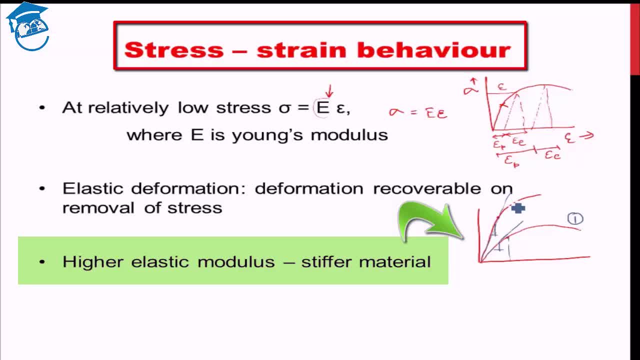 material is this slope. This is steeper. This is a steeper slope. That means the Young's modulus for two is more than Young's modulus for one, And the material which has a steeper Young's modulus more Young's modulus, means it is a stiffer material. What does that mean? 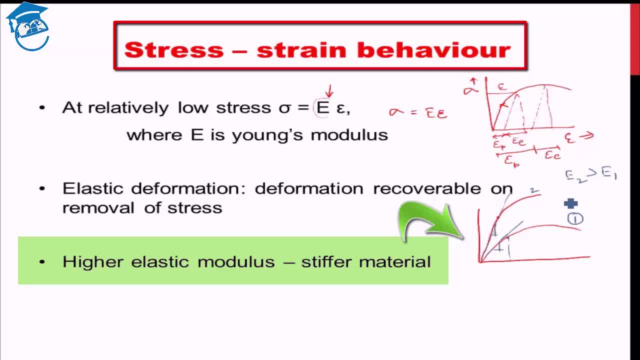 That means that to bring about the same amount of change in dimension, a stiffer material will require more stress. How can we say that- Let's mark this point- same amount of deformation: This, the first material, requires only this much amount of stress, whereas the second. 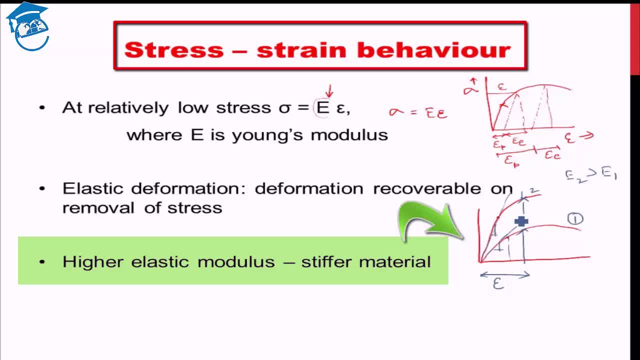 material requires much more stress. Therefore, the second material, which is a higher Young's modulus, is a stiffer material. Normally speaking, ceramics are more stiff material. they will have a much more drastic Young's modulus. Metals have shallow slope over here. thereby 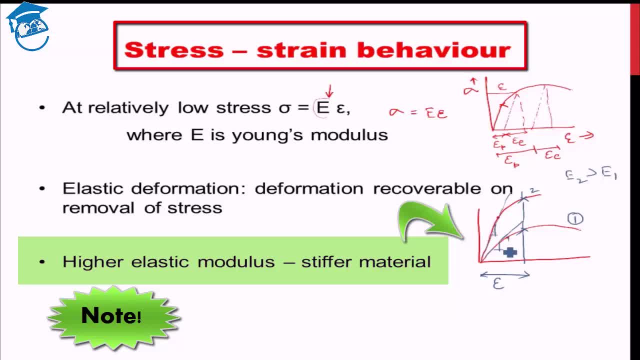 they have smaller Young's modulus compared to ceramic materials. In addition, ceramic materials only have plastic deformation. They have none of these deformation, These deformation or negligible elastic deformation. Therefore, what will happen if you have a ceramic material, the behavior, the stress, strain behavior for a ceramic? 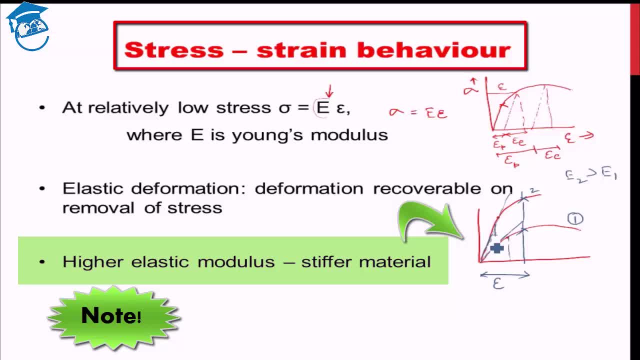 material will be something like this: It has a very high Young's modulus and just with a slight amount of plastic deformation it fractures. So the total amount of elongation that a ceramic material can go is quite less compared to a metal, But the Young's modulus is much higher. 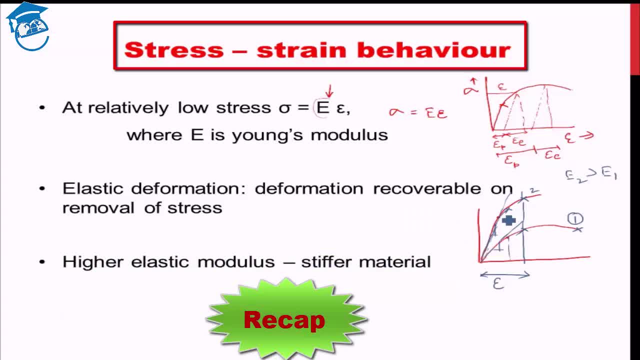 So what we have seen in this slide, just to recap, is that we have this proportionality, that is, stress is proportional to strain, linked by the Young's modulus. constant Elastic deformation is the amount of deformation which is recoverable on removal of the stress and higher elastic modulus. 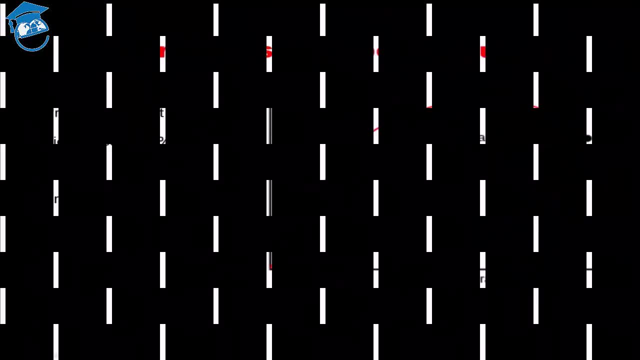 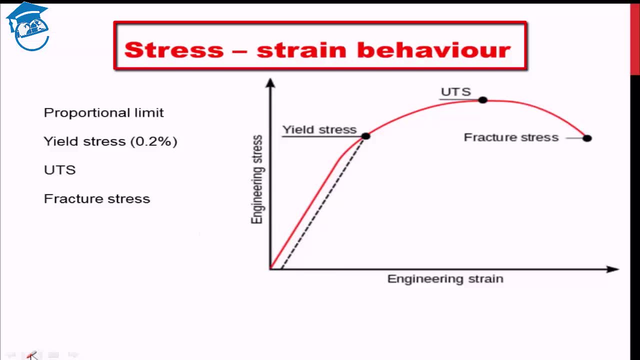 means stiffer material. Now let us see the stress strain behavior in details. This is a typical stress strain curve for a steel sample, mild steel kind of material Or aluminum, for example. mild steel will have a different behavior, or rather, other steel materials might have a different behavior. 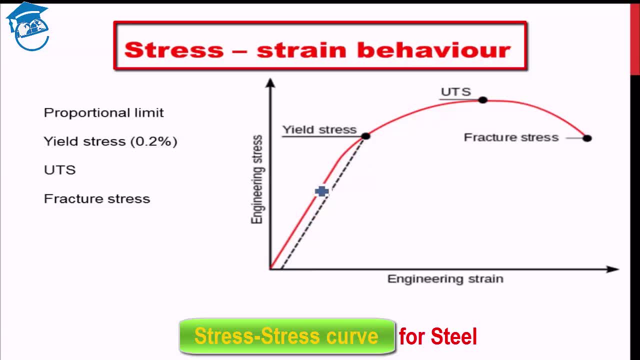 but this is more of a mild steel kind of behavior. In this. what we see is that we have something known as yield stress, ultimate tensile stress and fractured stress, and in addition to that there will be what I have said as proportional limit. Proportional limit is the position where the proportionality 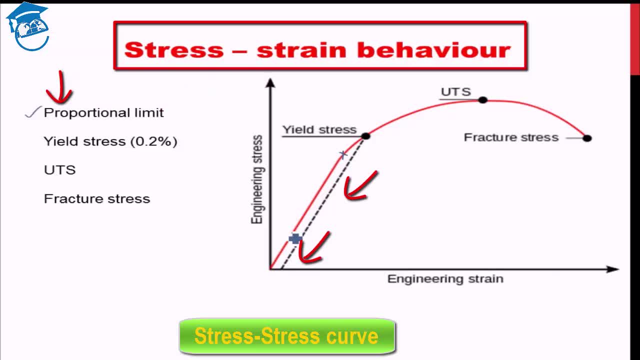 ceases to exist. Till here stress is directly proportional to strain. Over here the stress strain linearity deviates. but this two points are more or less always very close to each other. Since the proportionality limit, it is very difficult to identify exactly where the proportionality limit exists. 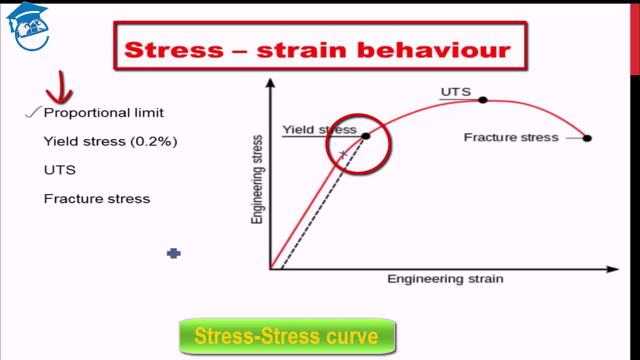 because, on a microscopic level, there might be that the stress and strain linearity ceases to exist, So this proportional limit is very difficult to establish. Therefore, what has been done is that we have defined a point known as the yield stress, which has been found out to be more or less the location. 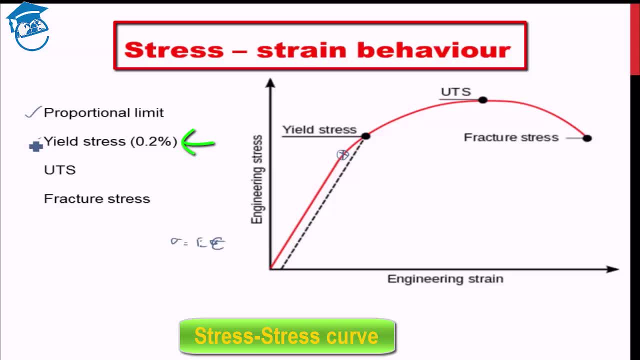 roughly where the linearity ceases to exist, But this has been defined as the 0.2 percent elongation region. So when the strain becomes equal to 0.002, that is the location. or this is 2 percent, that is the location, rather 0.02.. 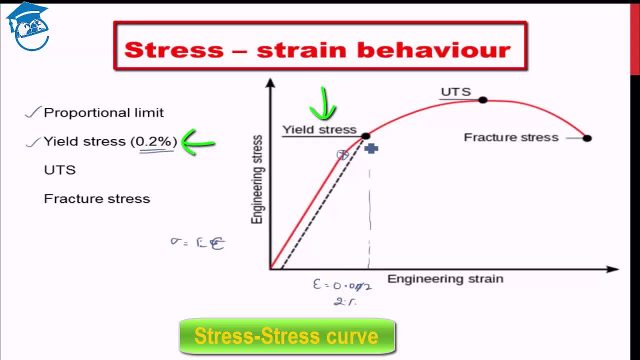 This is the location where we have yield stress. Beyond this, Plastic deformation starts. In fact, plastic deformation starts beyond this, But since these two will be quite close and this is not practically possible, we assume that yield stress beyond that, plastic deformation starts. Plastic deformation keeps on taking place, taking place. 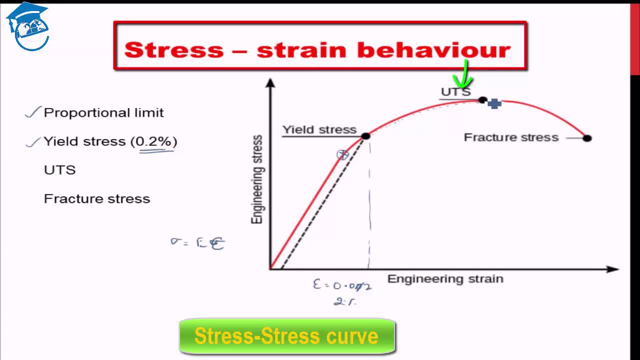 And finally, the ultimate tensile strength reaches when the necking starts. Necking starts here. and then what happens? When, at a lower stress level, the material keeps on elongating, the strain keeps on rising and ultimately, there will be fracture of the material somewhere down here. 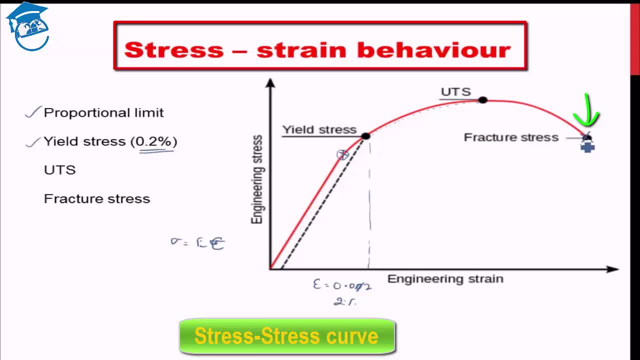 That is the fracture stress. The fracture will occur. Fracture stress is lower than ultimate tensile strength. Ultimate tensile strength is the maximum stress that a material takes, Max stress. Okay In the engineering Stress engineering, Engineering strain curve. 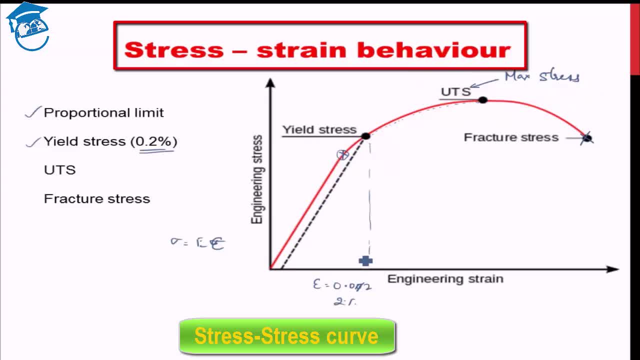 Just to clarify a point: In the yield stress I have said that it should be 0,, 2 percent elongation. This is the plastic right, The plastic elongation. Therefore, this is the actual 0.02 region. This much elongation needs to take place. 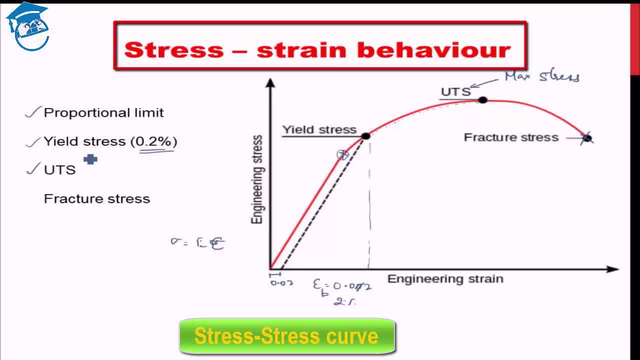 Fine, Now we have an idea about what proportional limit is, what yield stress is, what ultimate tensile stress or the maximum stress. What is the maximum stress value that a material can take handle is, and what is the fracture stress? Remember that all these are engineering stress. 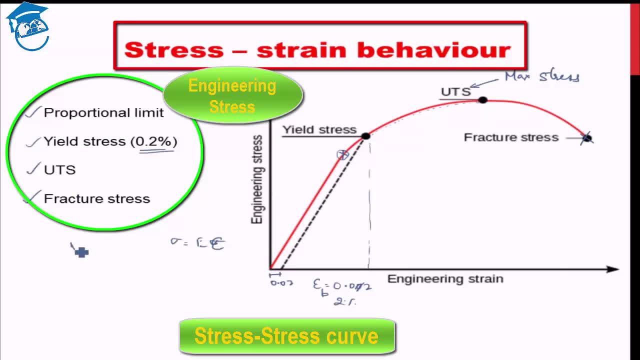 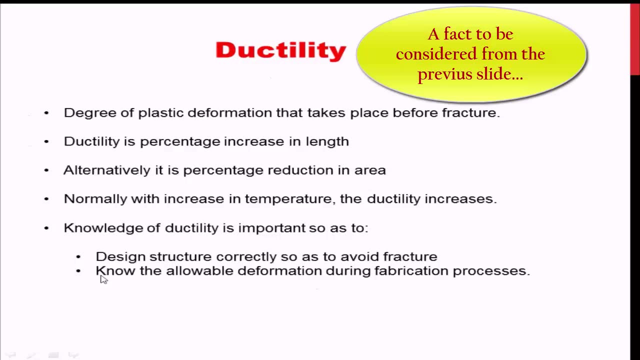 That is, the load upon the initial area, Not the instantaneous area, but the initial area. Now let us see what is ductility With ductility, With ductility. So this idea you have seen here that there is elongation taking place in the material, 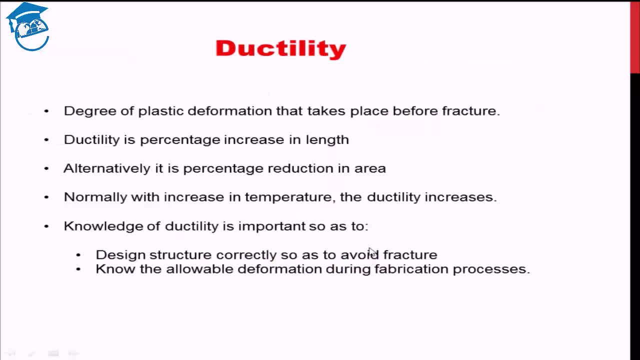 The material is getting elongated. So that amount of elongation, the amount of plastic deformation that a material can handle before fracture, is kind of indication of the ductility of the material. The other way to put it is: ductility is the percentage of increase in length that a material 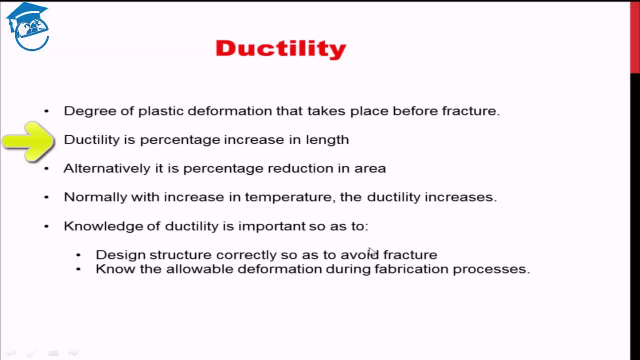 can have before fracture Or before failure. Okay, Before failure. Also, we know that the volume remains constant. right, Volume of material remains constant, So area into length remains constant, Since we are seeing the change in length as ductility. alternatively we can say the change. 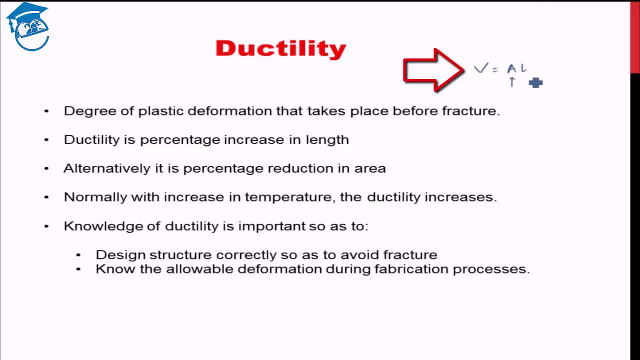 in area is also equal to ductility, But length is increasing, So increase in length is ductility, whereas reduction in area is ductility. Okay, Thank you. Normally speaking, ductility is something which increases with increase in temperature. Why is it so? 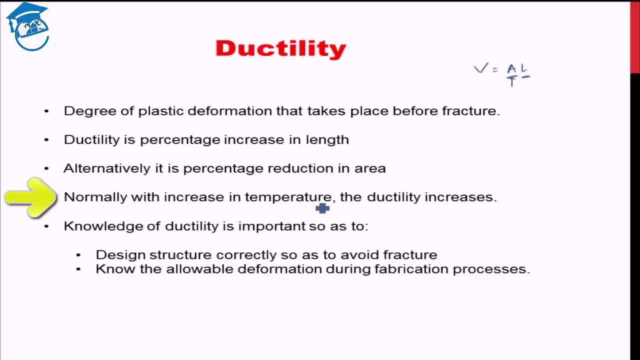 With increase in temperature, as we will see in details, the dislocation movement becomes easier, And dislocation movement is something which is very, very pivotal to deformation mechanisms. So easier it is for the dislocation to move, Easier it is for the material to deform. 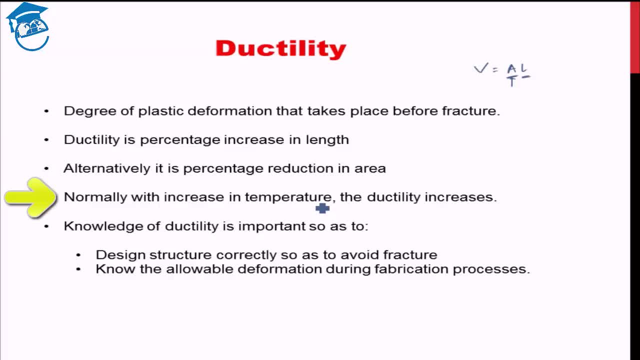 Thereby increasing of temperature leads to a increase in the ductility of the material, And the knowledge of ductility of the material is quite important. Why so? First and foremost, it helps us design the structure correctly so as to avoid fracture, If we know that a particular steel, let's say a steel A, can elongate maximum to 20%. 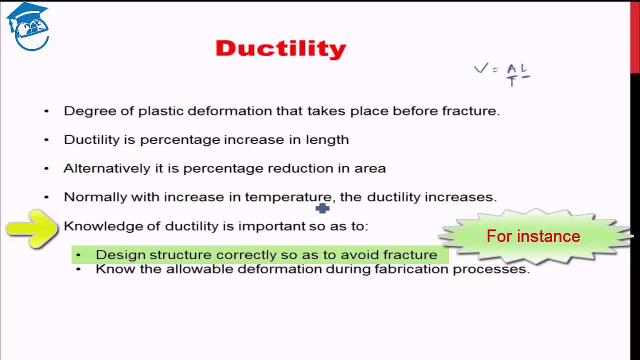 then we will design our material in such a way that the elongation of the material is less than 20%, so as to avoid fracture. Also, the ductility- the amount of deformation that can be possible in a material before fracture- helps us identify the allowable deformation during fabrication processes. 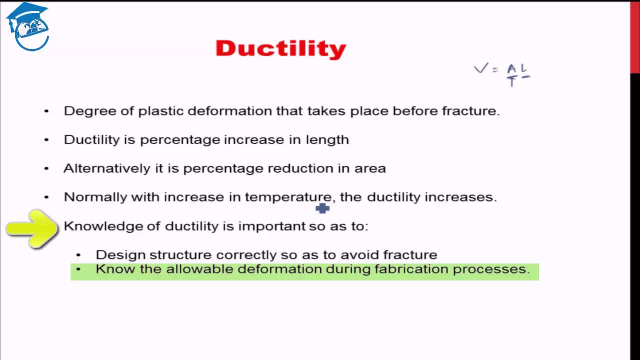 Right. There are many fabrication processes in which basically what we do is we let the material undergo plastic deformation. So if we know what is the ductility, we can estimate how much plastic deformation can the material undergo Thereby. ductility is an important parameter on those aspects. 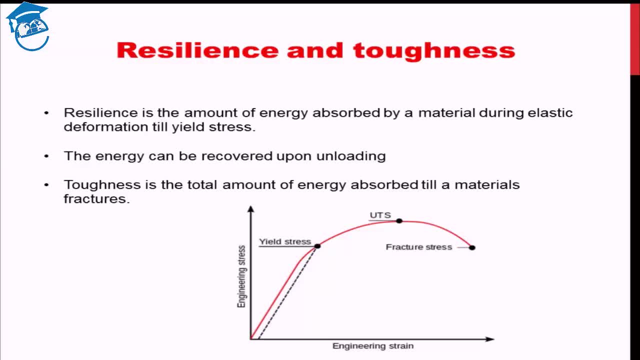 Now let us see what is resilience and what is toughness. The two terms, resilience and toughness, are related with energy Resilience and toughness. Resilience means the amount of energy absorbed by a material. Resilience means the amount of energy absorbed by a material. 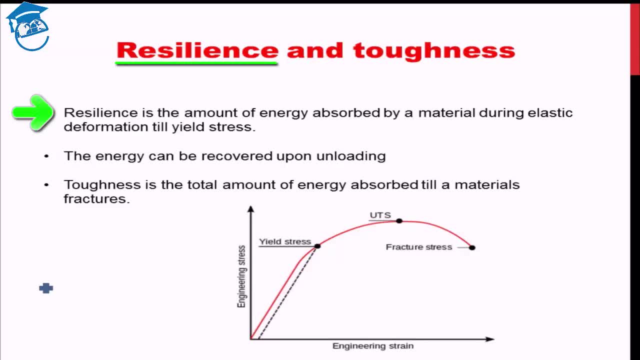 material during plastic deformation till yield stress. So resilience is basically area under the curve here. This is the resilience till yield stress, And the same thing is if we consider the toughness, then the toughness is the amount of energy absorbed till failure. Okay, 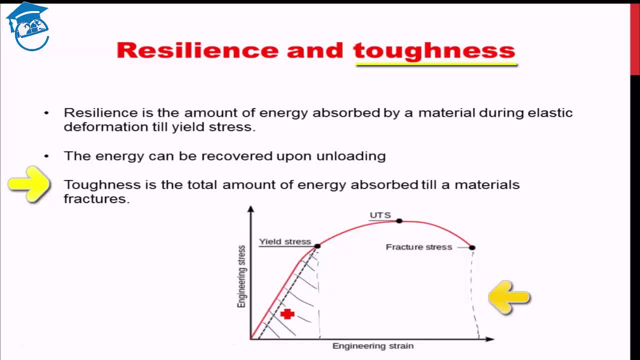 It is the amount of energy absorbed till failure. Okay, It is the amount of energy absorbed till failure. So this whole region is toughness. Resilience can be recovered upon unloading. Toughness is not recovered. Toughness- a part of it will be recovered, but not the whole. 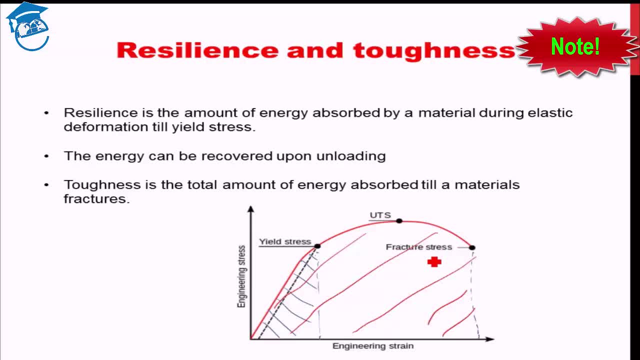 Okay, Toughness gives you an idea about how much energy can the material absorb before fracturing. Therefore, this is very important in practical scenarios. That is, how much impact can it take right or during crash of a vehicle, how much energy? 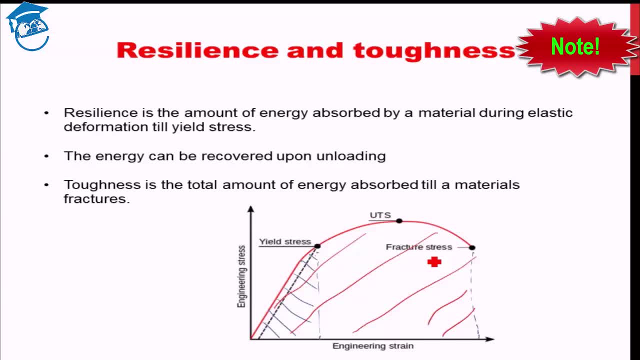 can it absorb before crushing and failing During strong winds? how much energy can the bridge take before collapsing, such kind of things? Resilience, on the other hand, tells how much energy can the material take before plastic deformation starts taking place. That can be very important in applications, because you don't want a material such that. 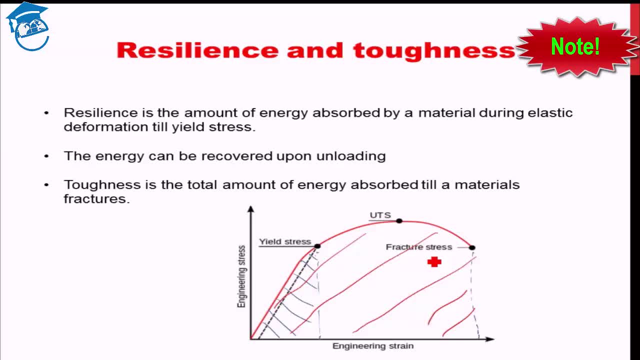 during application it starts to change dimension. So what you need is: during application the material has. the material specification is such that the energy it can absorb, it needs to absorb, is less than the resilience. else, if it is more than the resilience, then it will start to plastically deform and go out. 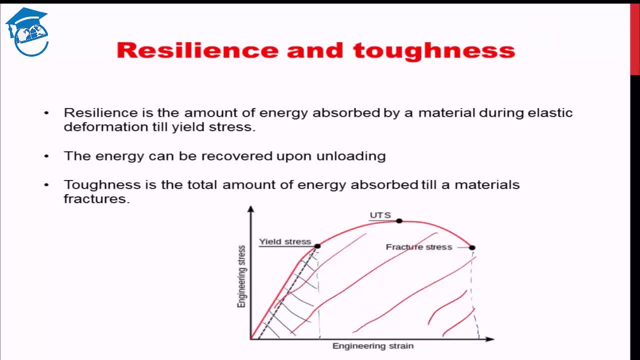 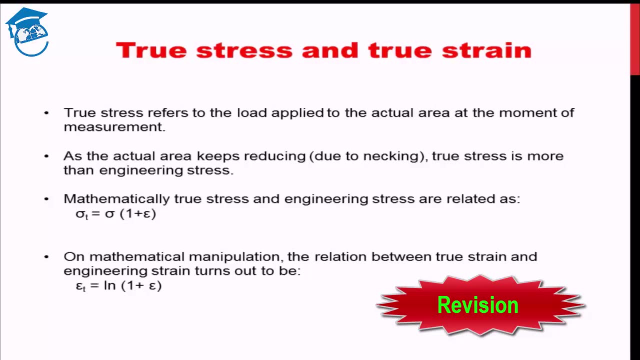 of shape. Okay, Now, with this idea about the energy requirement for transformation and deformation, let us revisit our concept of stress and strain. Initially, in the previous lecture, we discussed about engineering stress and strain, in which what we had is engineering stress was force upon initial area. right, 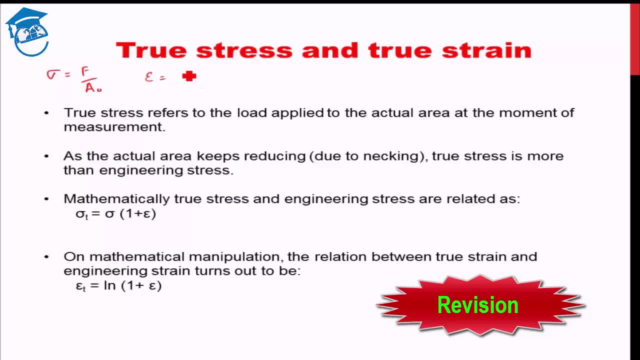 And engineering strain was change in length length, final minus initial length upon initial length, Whereas I said that true stress and true strain includes the idea of instantaneous area and instantaneous length. Okay, This is quite important. Why so? Because, in reality, during stress test, during tensile test, the area is continuously changing. 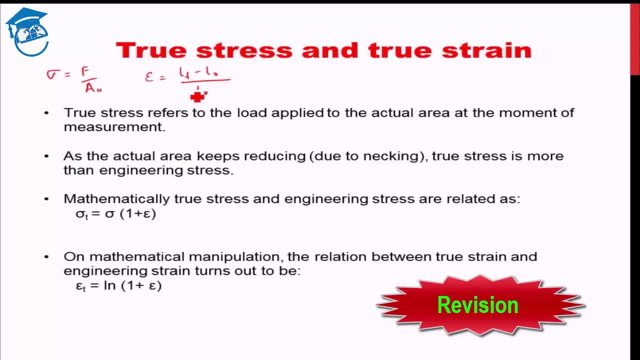 the length is continuously changing. Okay, So in reality, actually the amount of load being taken by the body is the true stress and the actual deformation is the true strain, not the engineering stress and engineering strain. So to complete the theory, we need to understand true stress and true strain too. 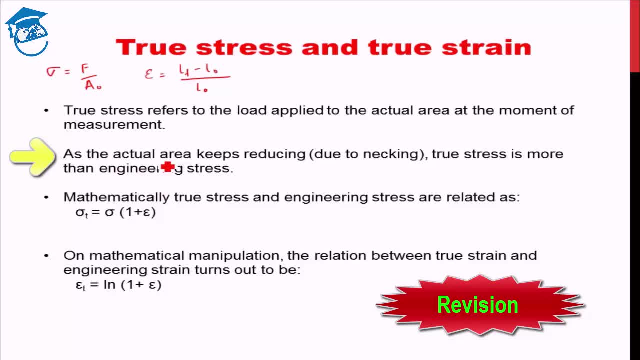 Okay, As I have said, in the actual area keeps reducing due to the necking. Therefore, true stress becomes more than engineering stress. Why? Because In this denominator, A is actually less than A naught, therefore engineering stress which will be sigma, let's tell E, F upon area instantaneous. 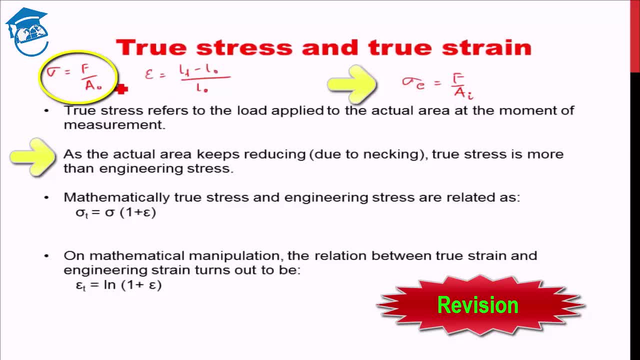 A I is less than A naught. therefore, sigma E is less than sigma right or sigma T. let us say sigma, true. Now on mathematical manipulation. what we see is that the true stress and engineering stresses are related like this: This is true stress is engineering stress multiplied by 1 plus engineering strain. 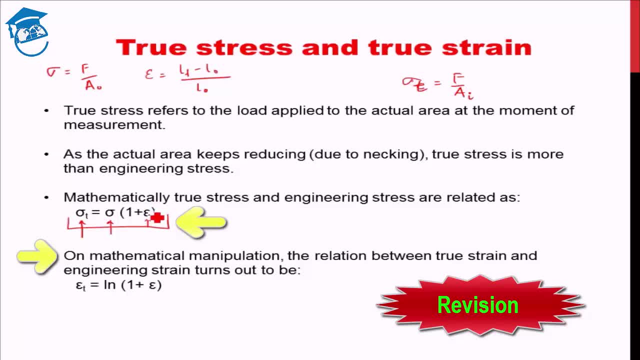 Okay, Since engineering strain is always more than 0,, this is more than 1, thereby the true stress is always more than engineering stress. Okay, We will not go into the mathematics of it. Just to give you an idea. I have shown you the relation. 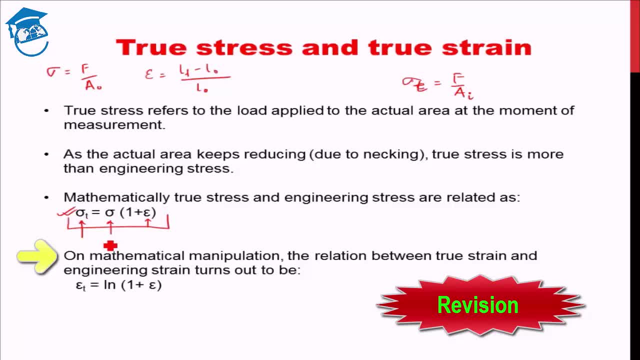 Similarly On mathematical manipulation, we find the relation between true strain and engineering strain, as true strain is natural logarithm of 1 plus engineering strain. Okay, Again, I will not go into the mathematics Now. with this we have come to the conclusion of today's lecture. 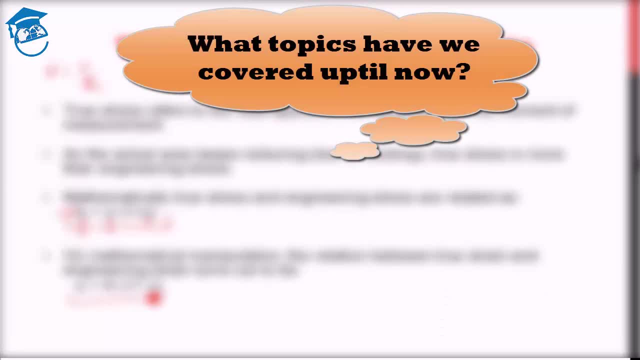 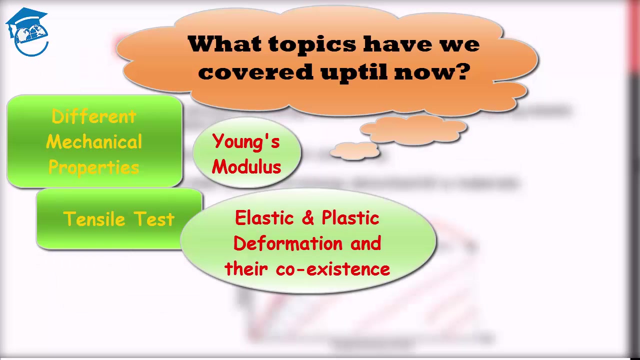 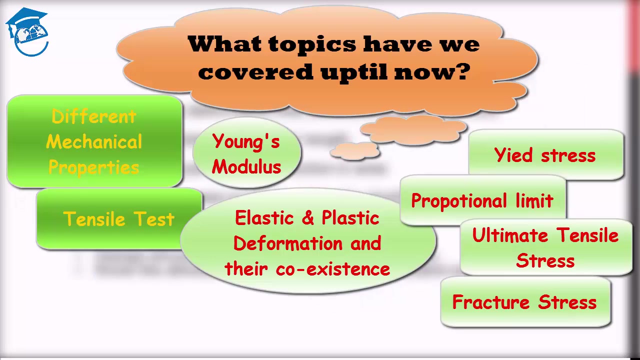 The previous two lectures, including today's lecture, we have discussed about the different mechanical properties. We discussed about tensile test. Today we saw the idea of Young's modulus. We saw how the elastic and plastic kind of deformation coexist. Then we saw the idea of yield stress, proportional limit, ultimate tensile stress, fracture stress. 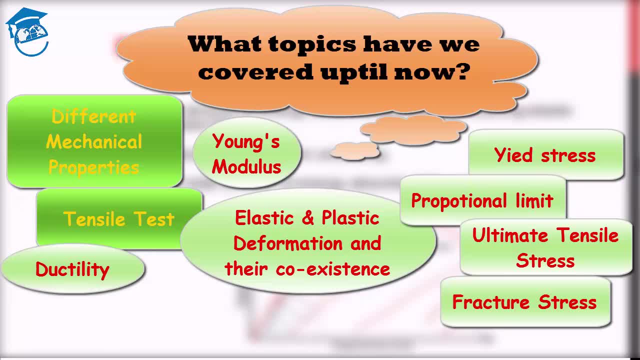 We visited what is ductility? we understood that Resilience and toughness that is related with the energy requirements. Then, finally, We conclude the discussion with the ultimate tensile, stress- Okay- And with the understanding of true stress and true strain.